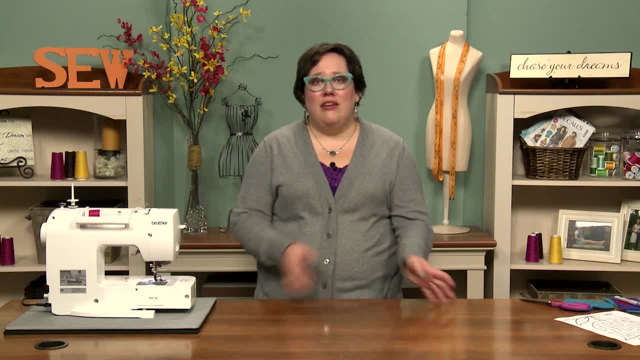 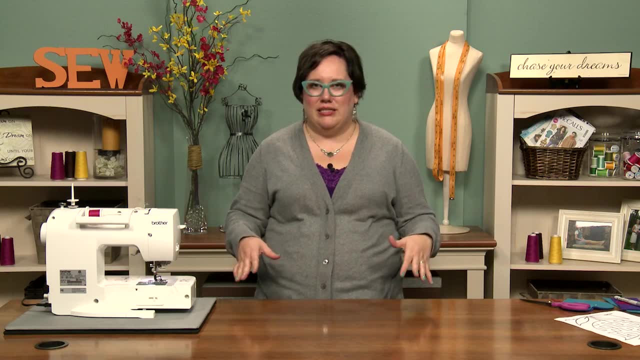 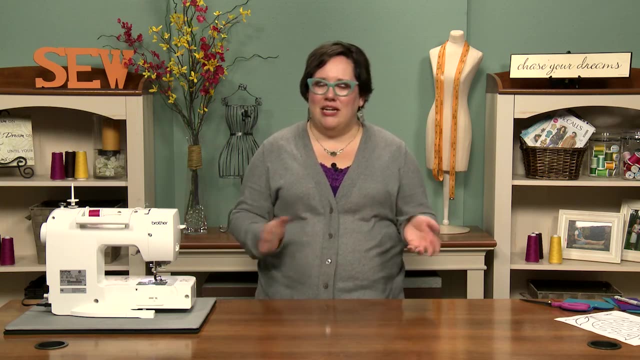 In addition to that, you want to make sure that, safety-wise, there's nothing going on outside of what you're doing. So try to get into a nice concentrated place where they're paying attention and you're paying attention to everything you're doing as you work together to sew a fun project or whatever you might be working on. 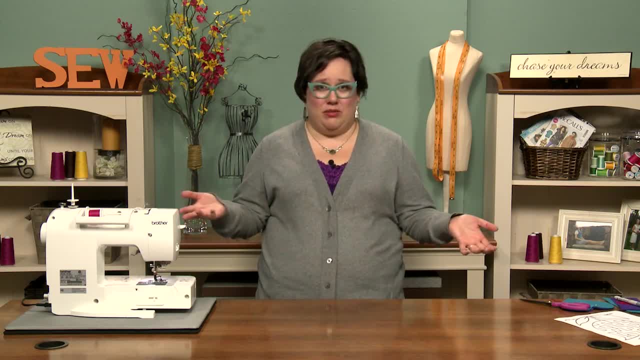 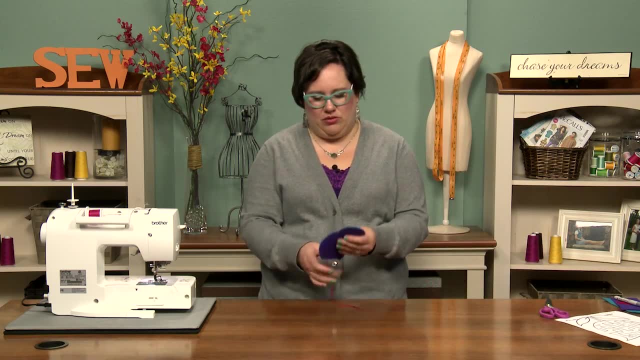 Now let's talk about some projects that you can get started with. I like to prep hand sewing first, especially with younger children, And I have sewn kids as young as well. I tried at one point a three-year-old who was very interested. 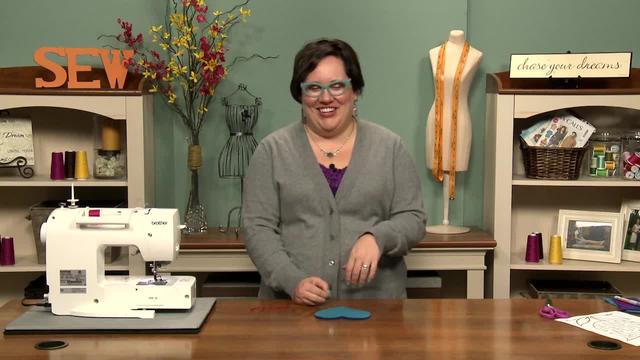 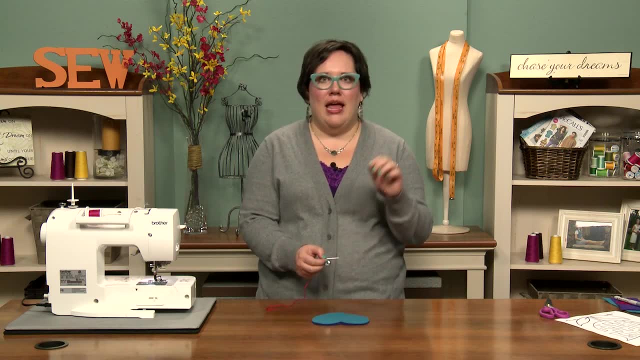 but eventually she turned four and that's when we really got started sewing together. So I like to you can get kind of kits that have a tapestry needle and yarn and a like a cardboard cutout that has holes pre-perforated in it. 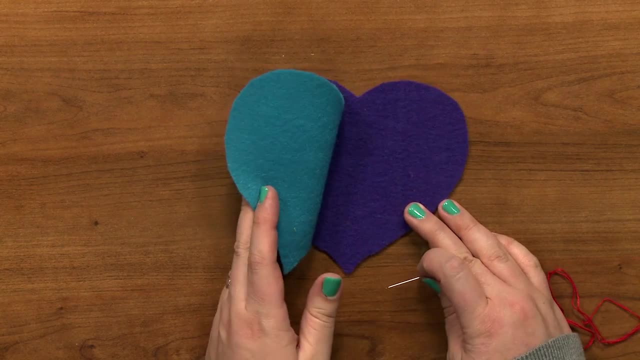 or you can make your own, which is what I've done. So I just have two pieces of fleece here and you can see that I have. it might be easier. nope, it's easier on this side. You can see that I've gone ahead and drawn it. 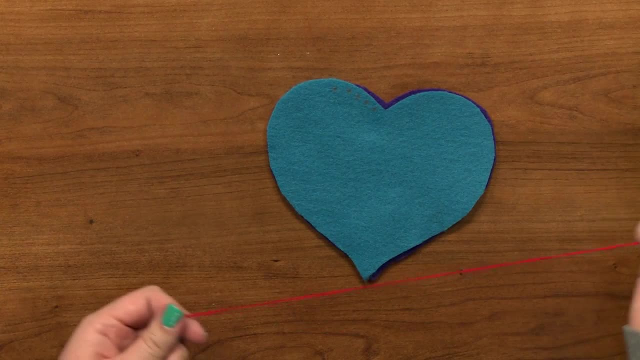 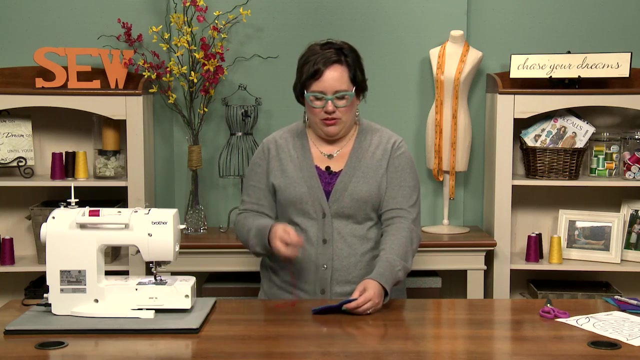 I've drawn a few dots on here to show where we should put some stitches, And then I've just knotted a contrasting color of thread. Of course, to get children excited about sewing you might want to show them. let them pick out all the colors and materials. 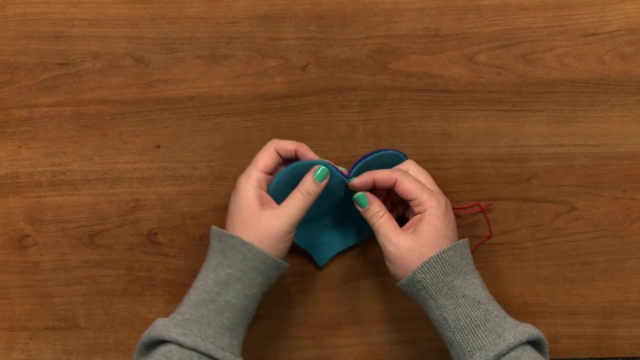 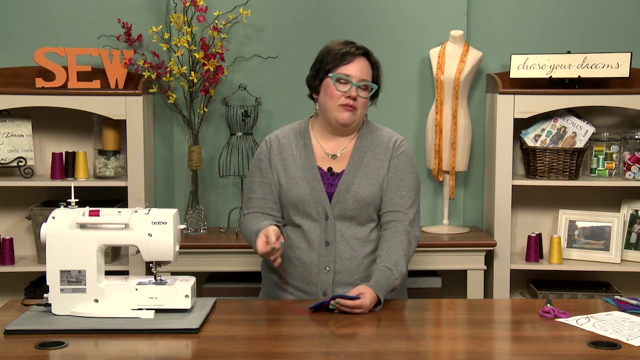 And then just show them this is how sewing works. You put it in at one dot and you come up at the next dot And they can learn this way. You know there's no, there's right ways and wrong ways of doing things. 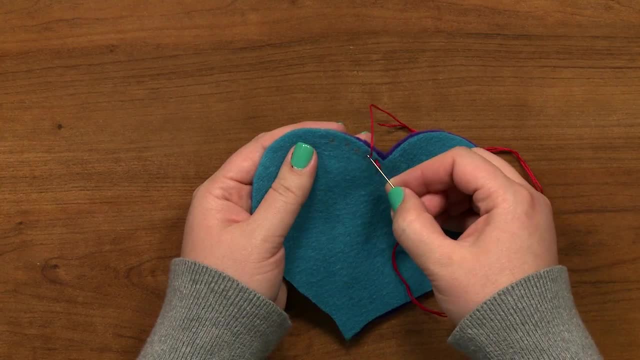 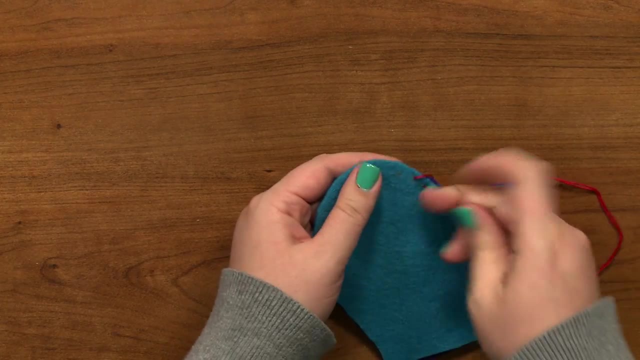 but when you're first starting out, it's mostly about the action of doing it. So you want to show them. you know, do it your way. but this is how stitches form, And I really like starting with hand sewing, especially on fleece or something along the or felt, as I have here. 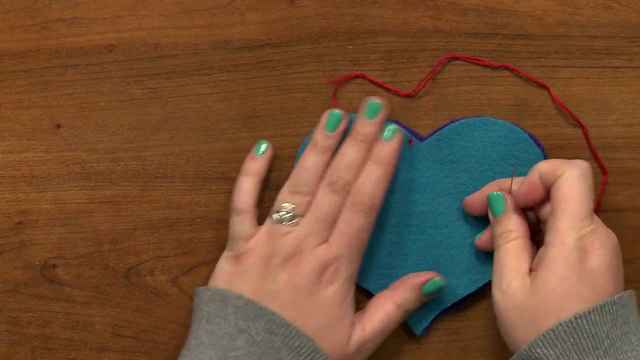 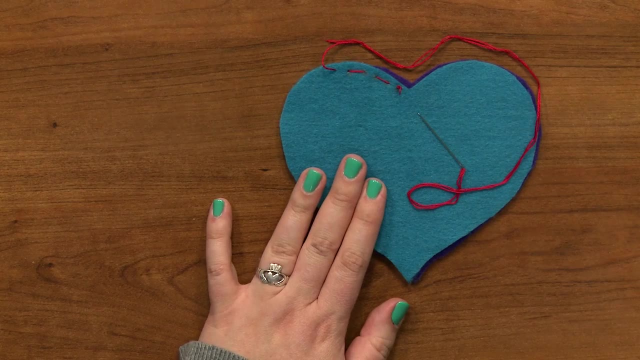 just because that's really easy to show them. you know, this is how sewing works. You're connecting two pieces of fabric with thread, You're making stitches, and it's either you making the stitch or it's the sewing machine making the stitch. 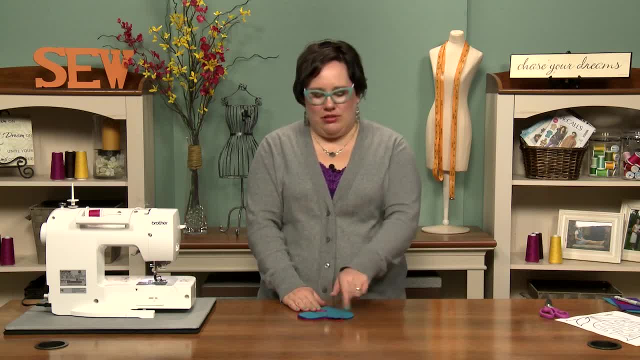 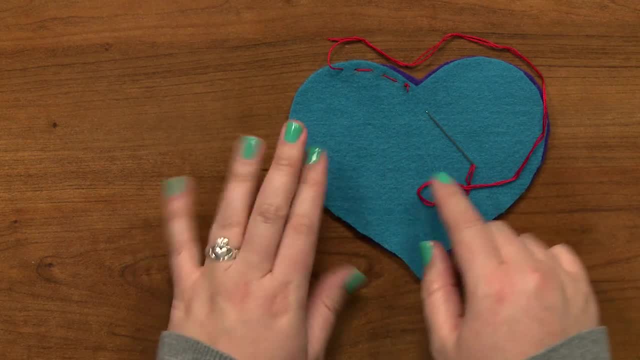 And I think this is a good way to get started, to show them how to sew this. Now, what kind of projects can they sew? Well, they could decorate the heart with thread, And then, in the middle, you could even write out some words for them to stitch over. 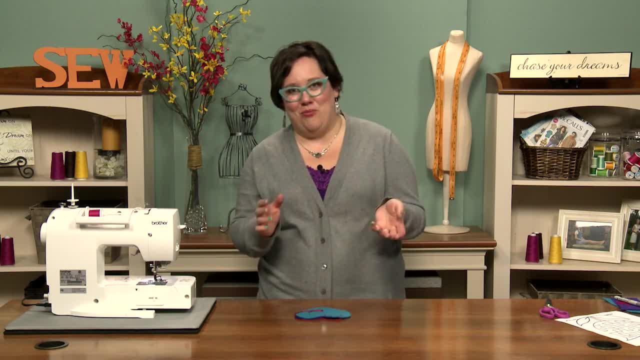 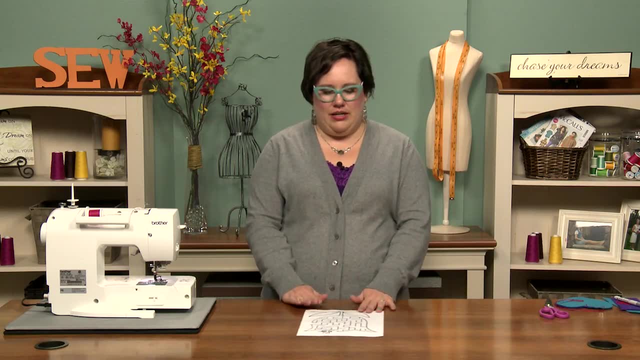 And that's a little Valentine they can give away or to put up on their wall. If you want to get started on the sewing machine, I recommend going online and just finding a coloring book maze. So I just searched for coloring book maze and I found this one, I believe, on Pinterest. 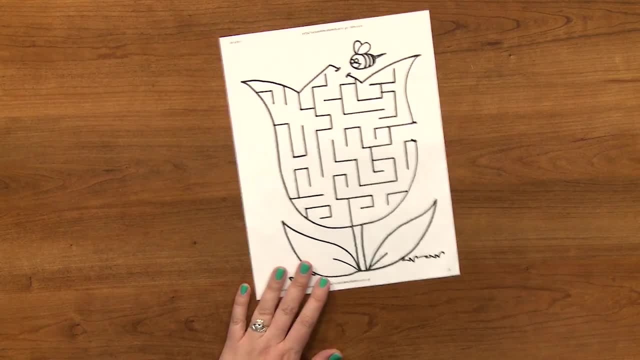 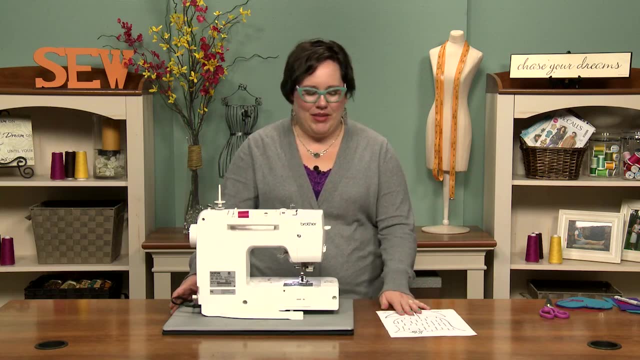 And it's good to have ones with big, wide, open lines, And this is a good way to kind of give kids a little bit of information about the safety of using a sewing machine. So we're just going to sew the maze as though we were doing it with a crayon. 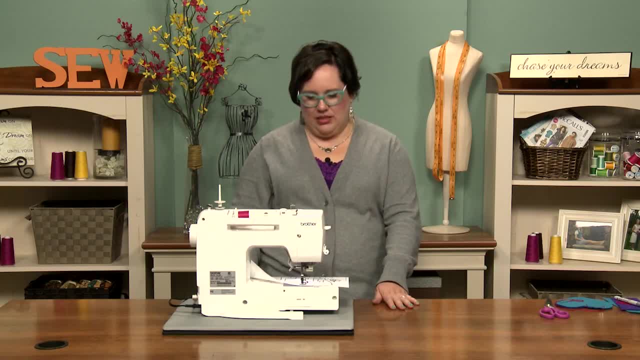 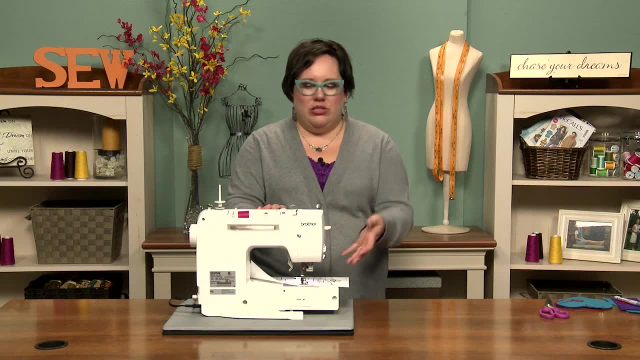 And here we're using a needle to sew paper, So that means that this needle is no good anymore. We need to only sew paper in the future with it, et cetera. So when you're starting out teaching a child how to sew on a sewing machine, 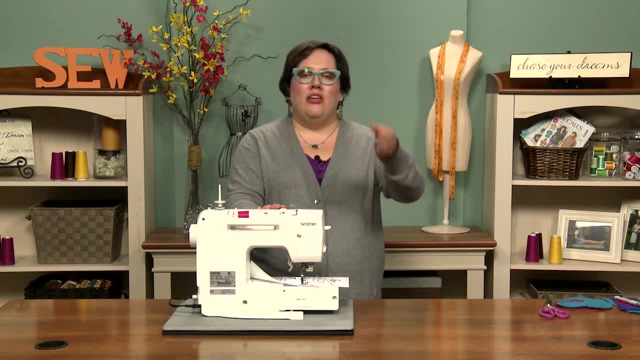 you want to teach them the parts and where the needle is and what's moving, You should demonstrate first how the machine works so that they know what to expect when it's running. And it may work out best if you use the presser foot and they move the paper around to begin with. 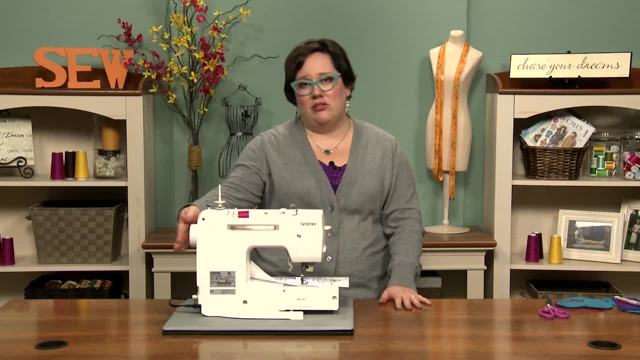 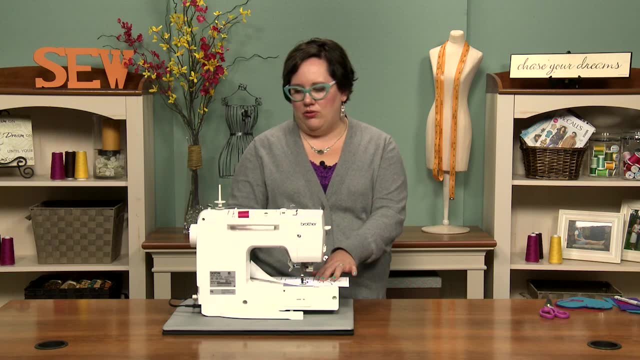 And then, once they're comfortable with that, they can use the presser foot. You can also always just instruct them to only use the hand wheel to go through the maze, which is also fine, because you could just go all the way through the maze using the hand wheel. 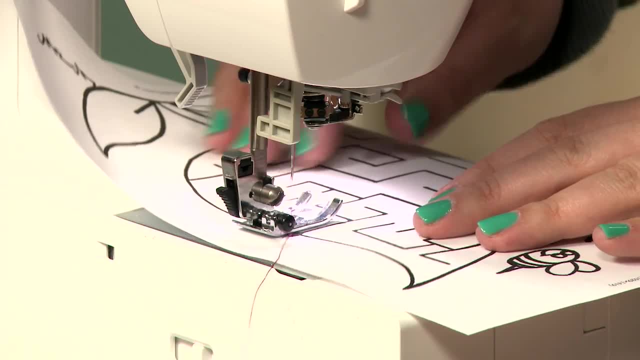 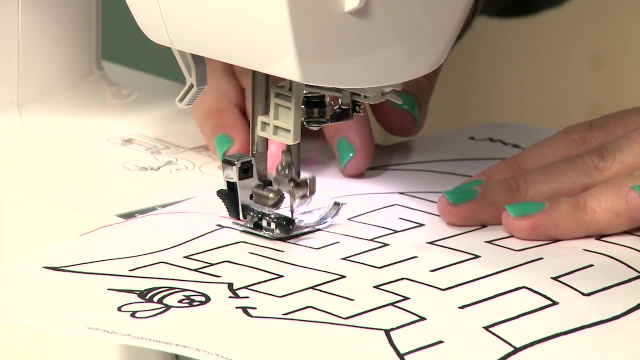 It would take a while, but you could certainly do it. So you would just sew around, And this is a good way to go, because it teaches them about pivoting and what to do when you get to a point where you're ready to go a different direction, right. 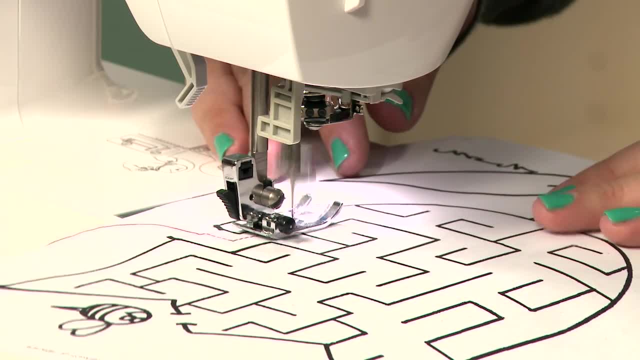 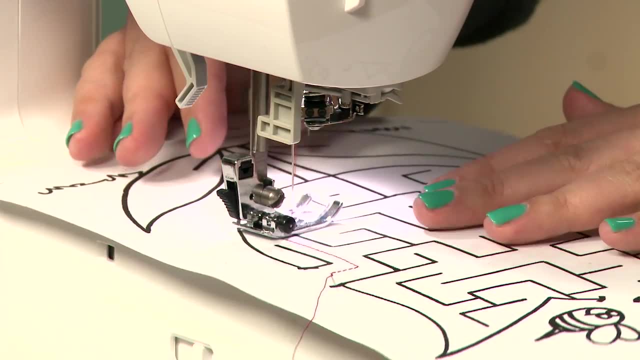 And you just kind of go through the maze and they can try to find the solution or they can try to find every possible route to go on the maze right. It's really easy and quick and simple. You can kind of show them when they're done. 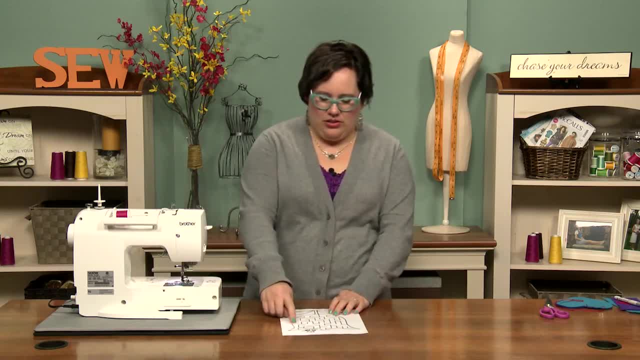 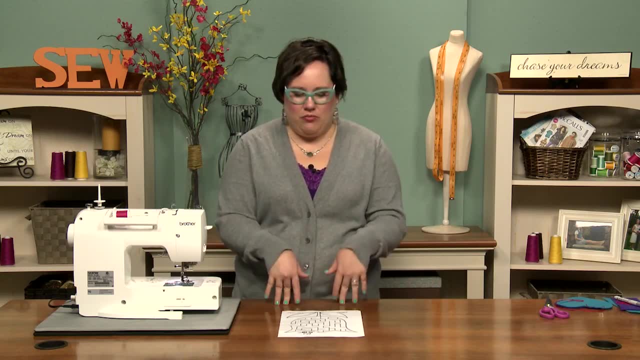 Okay, well, here's a spot where you pivoted really well and that looks good, but down here you started going a little crooked, And so you should. you know, here's how to work on that, And so this is a fun project, just to introduce kids. 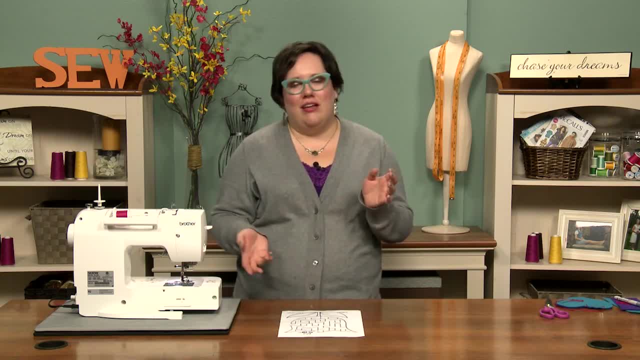 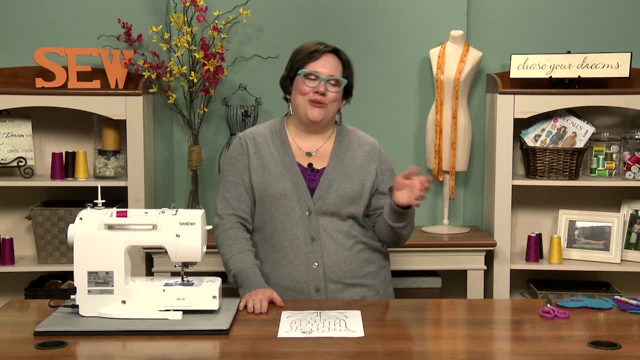 to the sewing machine is going through a maze together. I'm sure they'll love it and you'll enjoy showing them how to use the sewing machine. After that, I recommend letting them pick out the materials, because, of course, that's the most fun part.